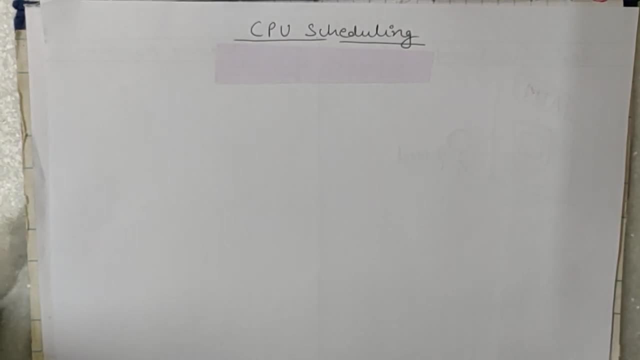 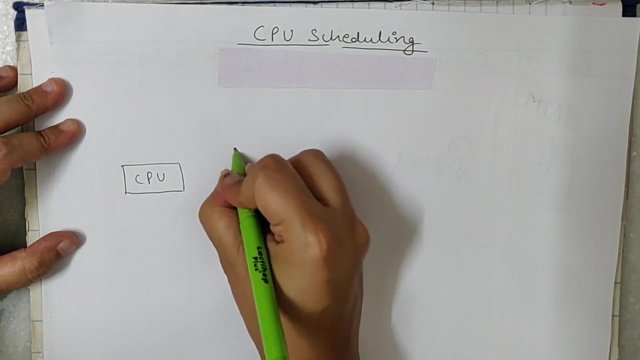 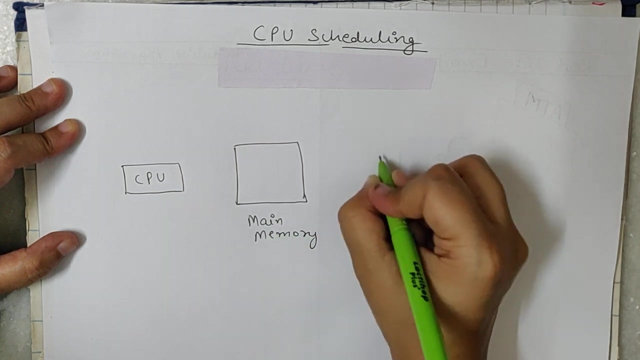 Hello everyone. The next topic in operating system tutorial is CPU scheduling. So let's understand why there is a need of CPU scheduling. Let's understand with the example. Suppose this is a CPU: Here is the main memory And here is the secondary memory. Okay, Secondary. 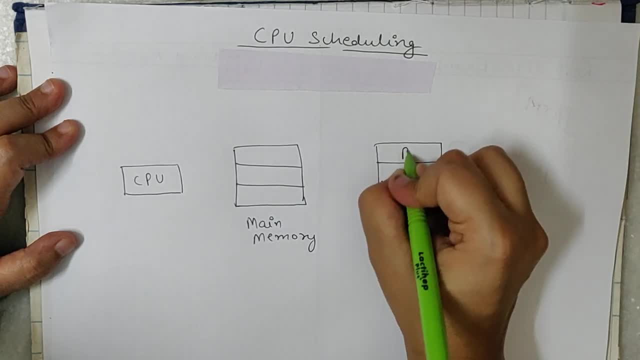 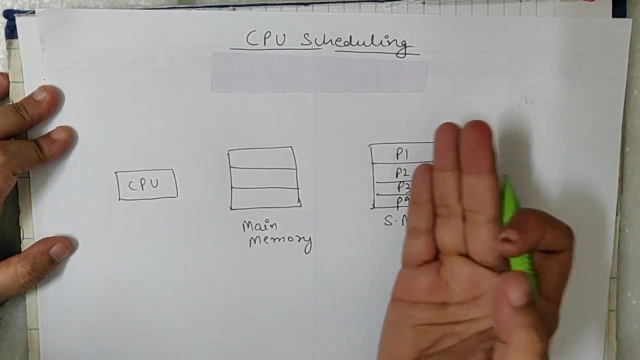 memory And this is main memory. Suppose I have a program- P1,, P2,, P3,, P4 and so on- in secondary memory And I want to execute P1,, P2, P3. So they has to reside in the main. 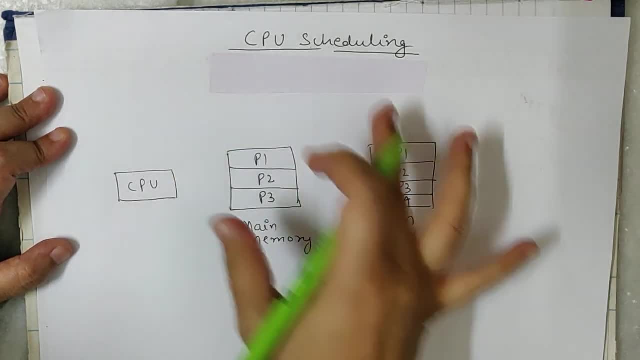 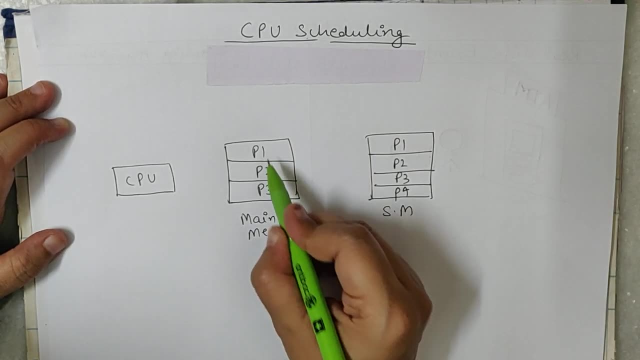 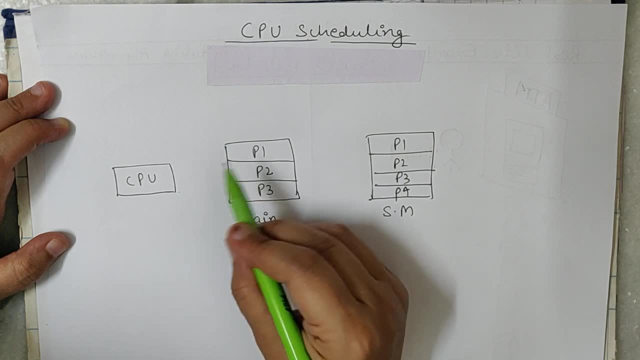 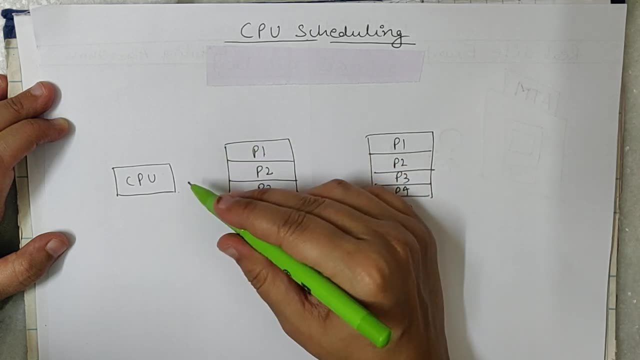 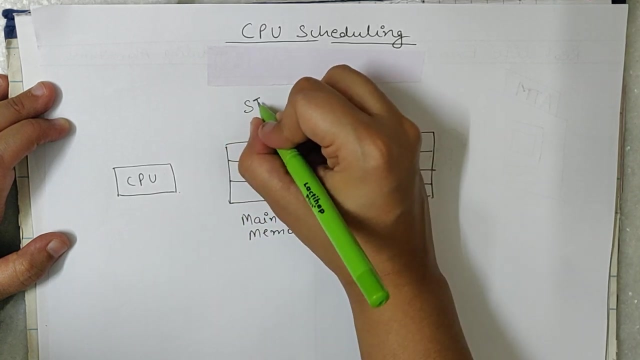 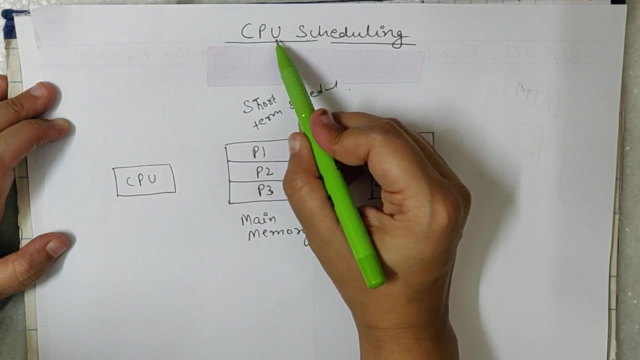 is only one, only one process at a time will get the CPU. Okay, So P1,, P2 or P3, who will get the CPU? Who decided Decide this short term scheduler? Okay, Short term scheduler. This is already. I have discussed short term scheduler And this is also known as CPU schedulers. 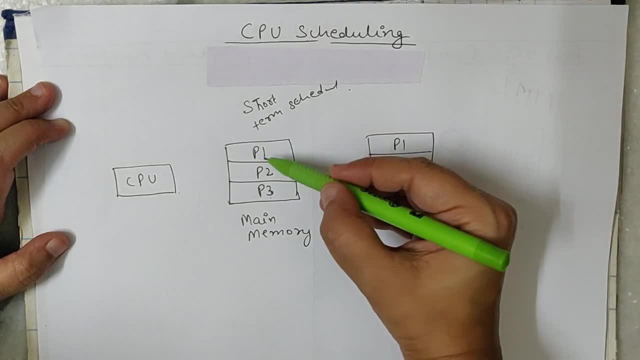 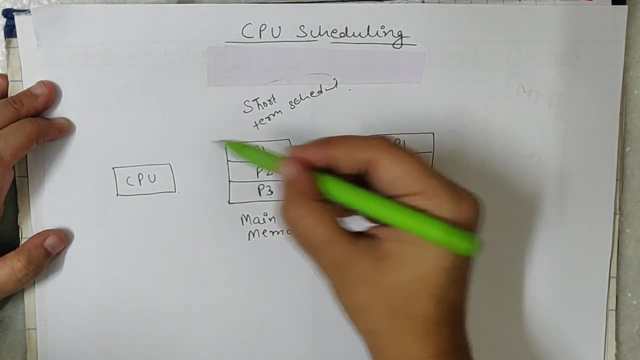 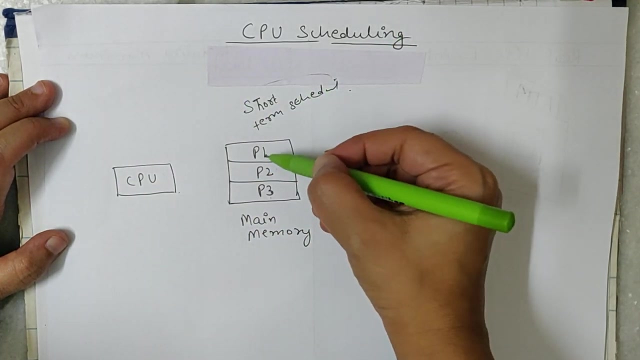 Okay, Short term scheduler are also known as schedulers. so what criteria short term scheduler will use? suppose i have said ki, p1 will get the cpu first. so how i have decided this short term scheduler, how it will decided that p1 will get the cpu first, on what criteria, on what basis it decides ki? 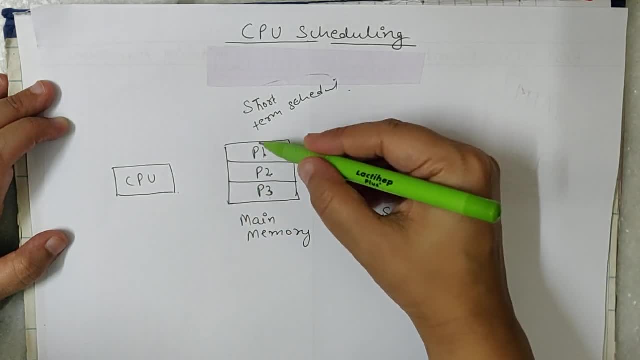 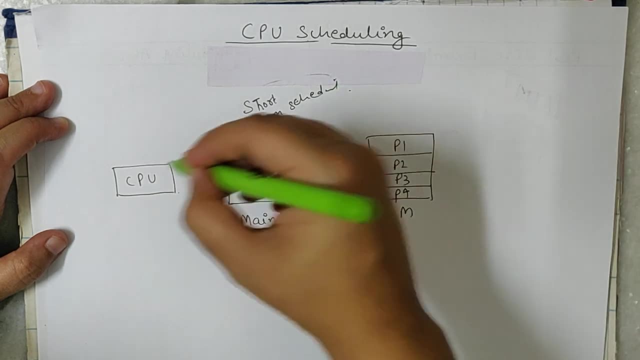 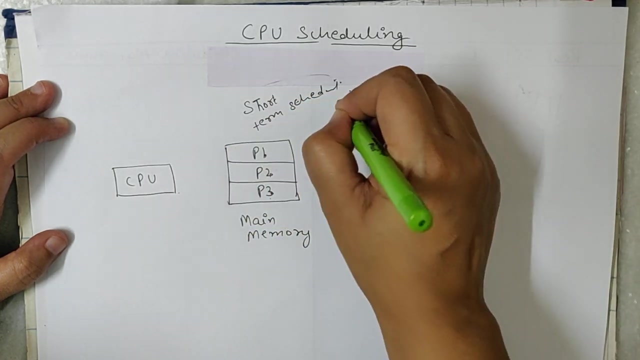 p1 will be discovered earlier in the cpu, rather than p2 and p3. why not p2? so p1, p2 and p3: who will get the cpu first and who will get the cpu later? so this is Information Controller and this is short term scheduler. but what basis is this and on what basis is? 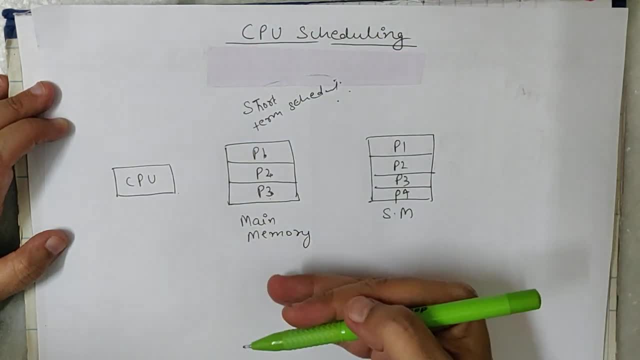 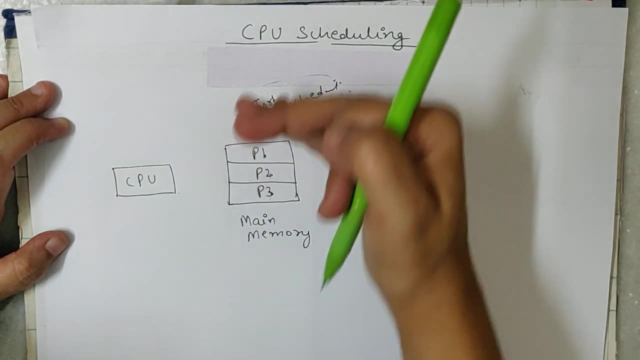 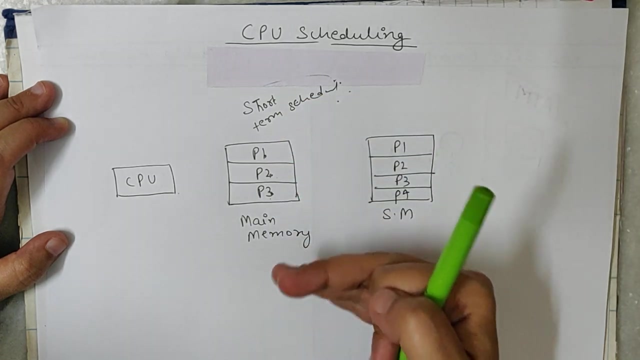 it decided. so this we call cpu scheduling. then İt means there is lot of processes ready in queue. All processes require CPU. but on what basis will we decide who will take CPU first and who will take CPU later? This is called CPU scheduling. 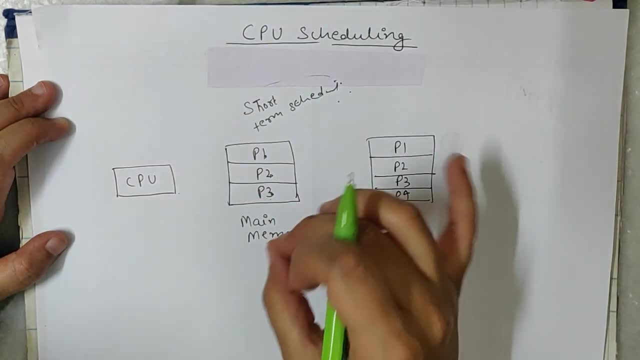 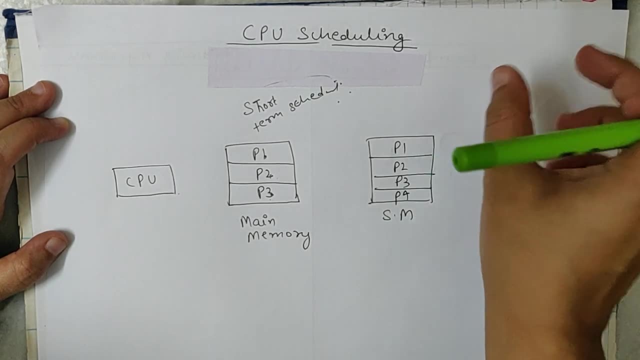 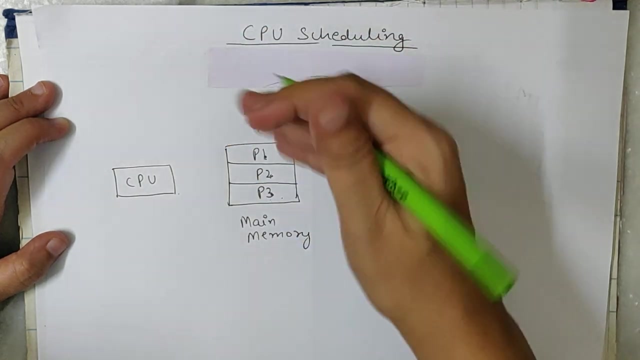 On what basis is it decided? This is all based on CPU scheduling algorithms. There are different algorithms and each algorithm has its own criteria. On the basis of those criteria we decide who will go first. So who will go first? There are so many processes in the main memory, in the ready queue. 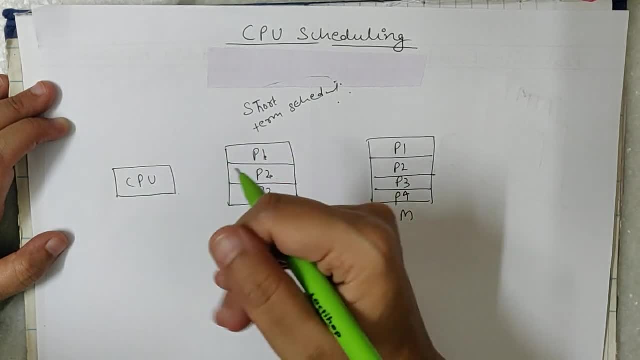 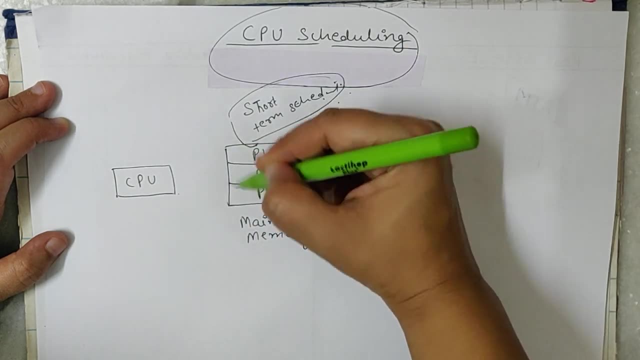 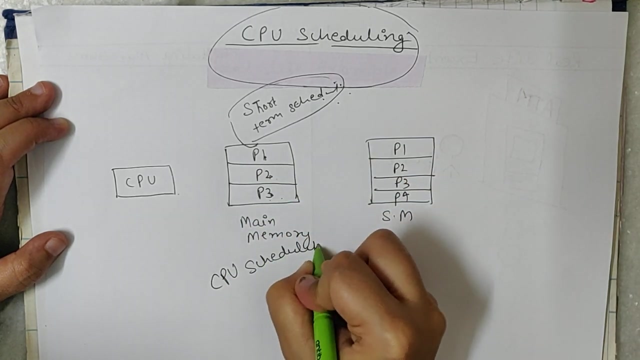 So who will get CPU first and who will get CPU later? This is called CPU scheduling. And who does this? Short term scheduler does this, But on what basis do we decide this? For that we have to use CPU scheduling algorithms To decide the criteria. on what criteria basis are we giving this particular process to the CPU first? 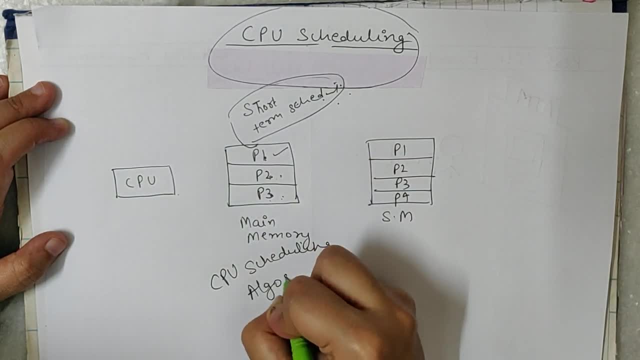 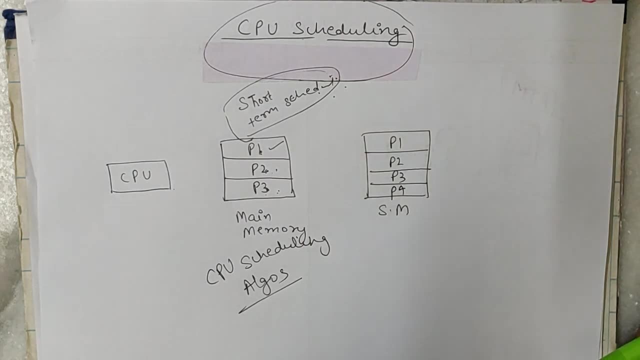 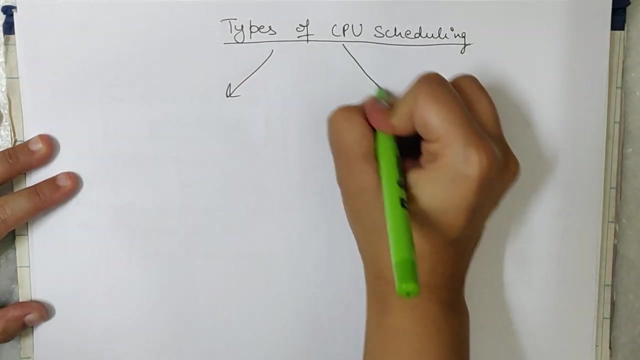 Or on what basis. These are CPU scheduling algorithms. So I will discuss the CPU scheduling algorithms with you. Before that, I will discuss the two types of CPU scheduling. So there are two types of CPU scheduling. First one is pre-emptive scheduling. 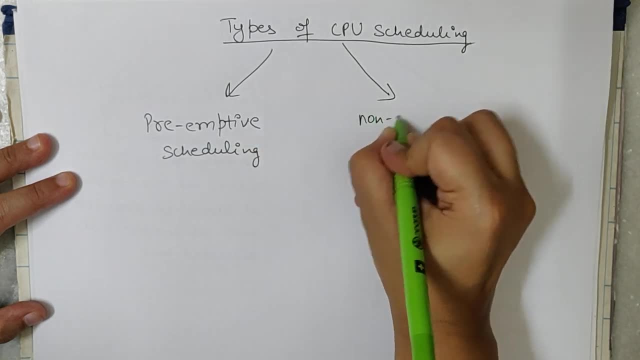 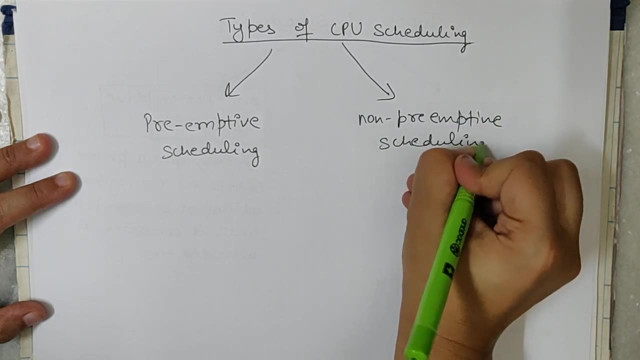 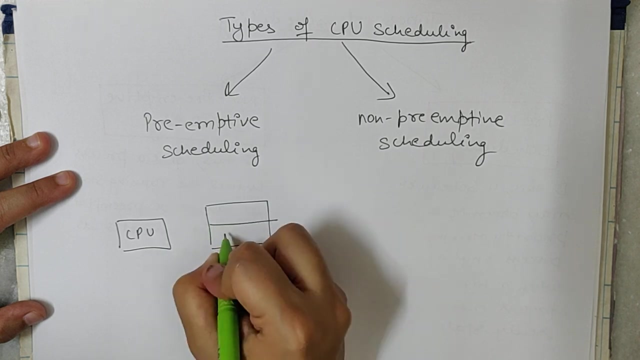 And the other is non-pre-emptive scheduling. Now let's see one by one what this means. Pre-emptive scheduling means this is CPU, This is the main memory, And suppose there are two processes in the main memory for the execution. 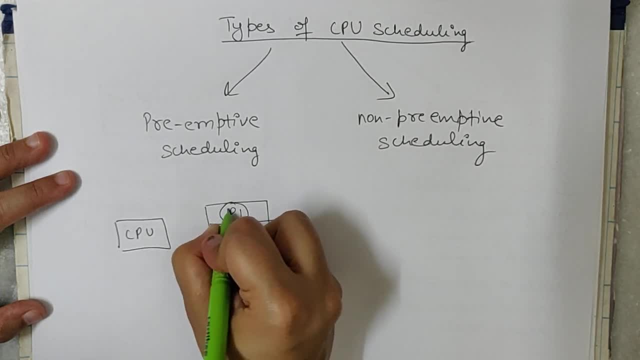 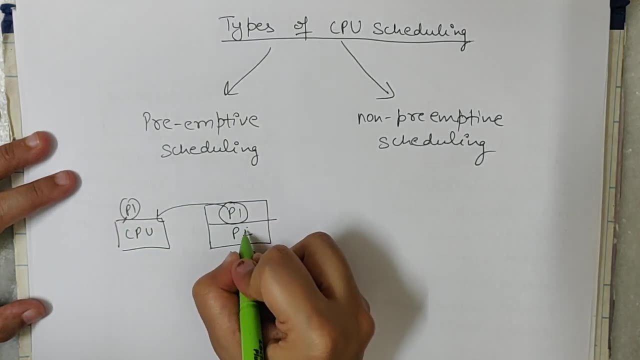 This is our main memory. Suppose P1 got CPU. P1 is using the CPU. Now suppose P2 comes in between. Its priority is higher than P1.. P2 has higher priority as compared to P1. So P2 in case of pre-emptive scheduling. 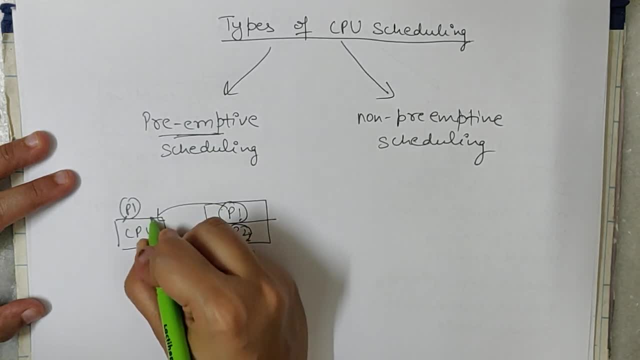 I am talking about pre-emptive scheduling. If P1 is already accessing the CPU and P2 comes with higher priority, P2's priority is higher, So P2 can interrupt P1.. It can remove it from here and will get the CPU. 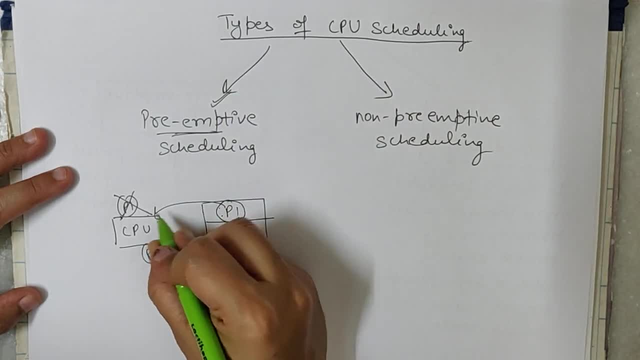 This is pre-emptive scheduling. If one process is already accessing the CPU And if another process comes with higher priority, Then the one which is already accessing will have to leave the CPU And the second P2 process will get the CPU. 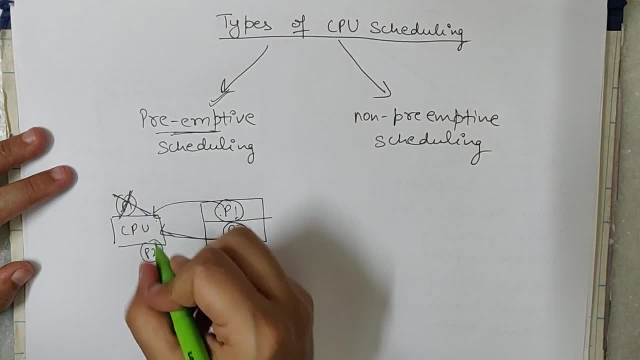 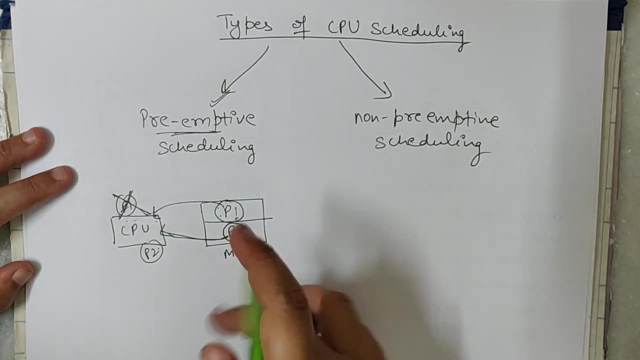 So P2 pre-empts P1.. P2 has pre-empted the CPU, P2 has removed P1 from the CPU And P2 will get the CPU. So P2 pre-empts P1.. Because P2 has higher priority. 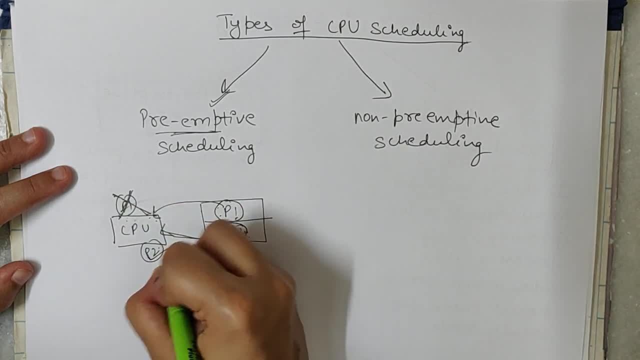 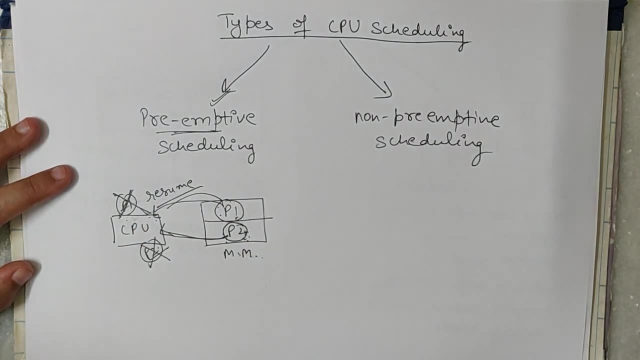 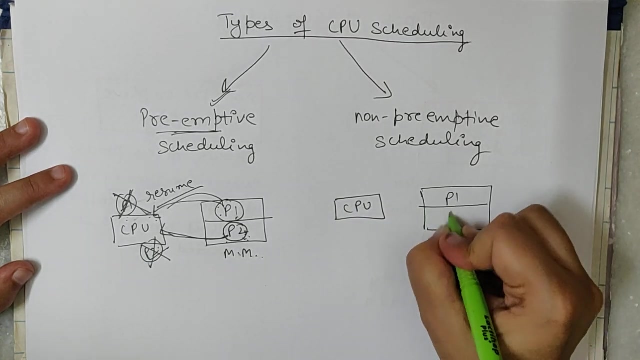 So P1 is removed from the CPU. When P2 executes and comes out, Then P1 will resume its execution. It will start executing from where it left off. But as compared with non-pre-emptive scheduling, What is there in non-pre-emptive scheduling? 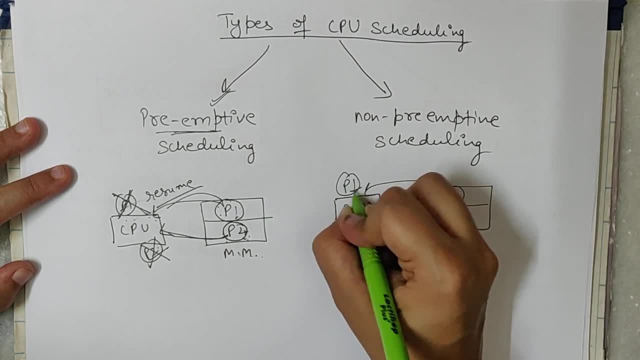 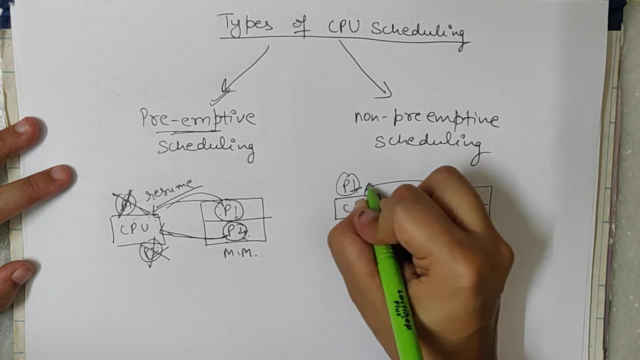 If P1 will get the CPU, P1 is accessing the CPU. If P2 is of higher priority, Then also it will not pre-empt P1. So P1 will not get the CPU until it executes it completely. This happens in non-pre-emptive scheduling. 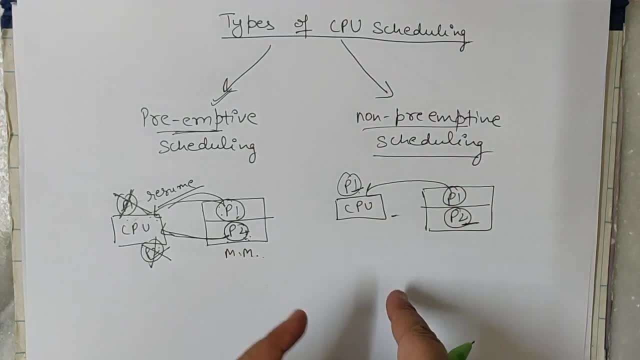 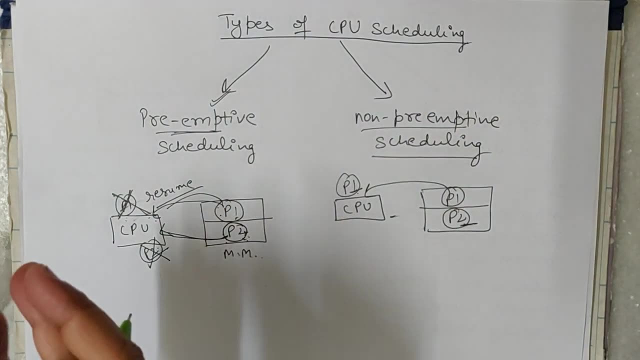 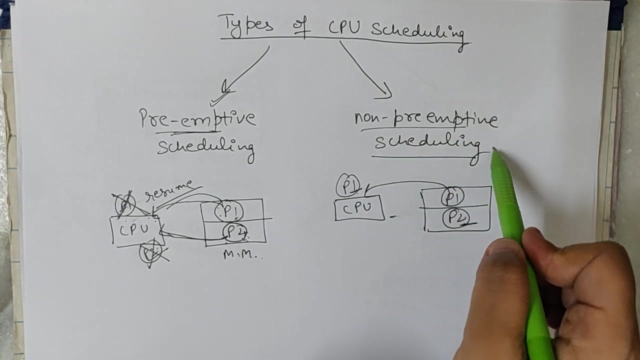 You cannot take over the CPU from the other process If already one process is executing the CPU. So these are the two types of scheduling algorithms: Broadly categorized scheduling algorithms: CPU pre-emptive scheduling algorithm and non-pre-emptive scheduling algorithm. 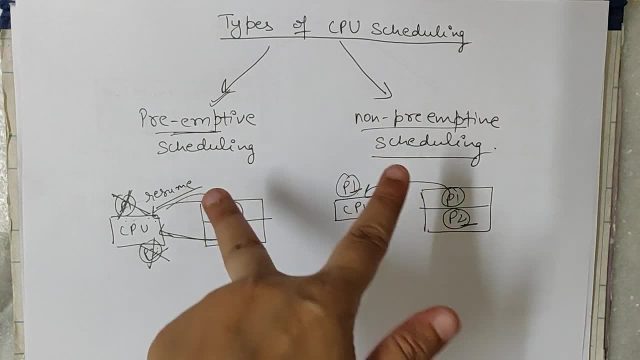 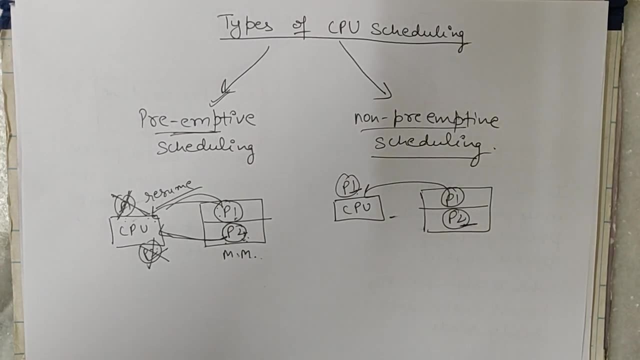 We have various algorithms, obviously, But these are the two broad categories: Pre-emptive scheduling and non-pre-emptive scheduling. I hope this is clear: The pre-emptive and non-pre-emptive scheduling. This is the formal definition of pre-emptive scheduling and non-pre-emptive scheduling. 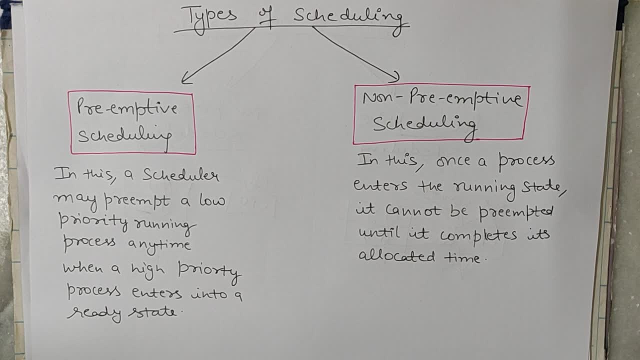 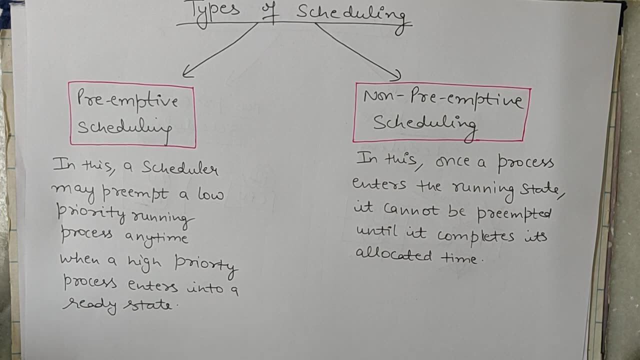 I have already discussed this, So you can take a screenshot. In the next tutorial, I will discuss the types of CPU scheduling algorithms. This is the broadly categorized. These two types are broadly categorized. Okay, And now under these categories, We will have different CPU scheduling algorithms.